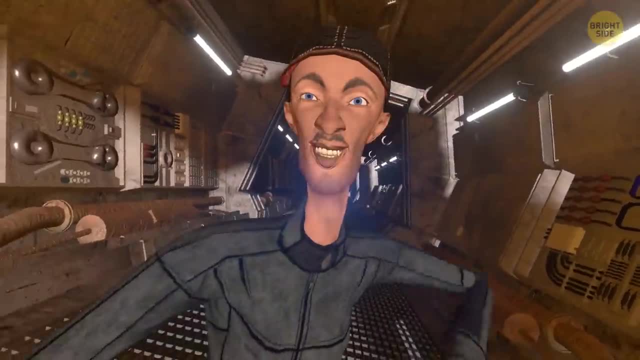 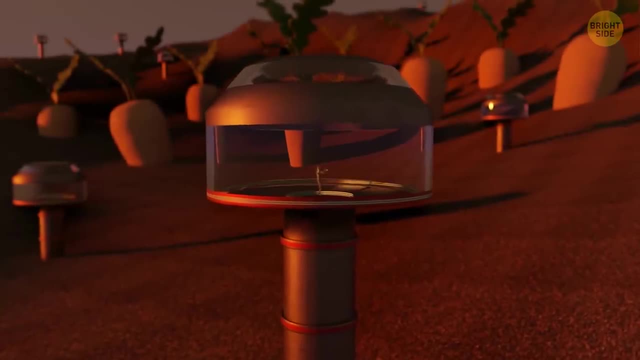 You might just need a whole new skin. How do you feel about orange? Sorry people, Green skin is totally sci-fi. Here's the deal. Carotenoids offer quite a nice protection against UV light. That's the stuff you find in carrots. Sweet potatoes, bell peppers, tomatoes, pumpkins- A Mars farmer's market could make a fortune. The more of these veggies you eat, the more orange your skin's gonna get. If you followed a special diet and wore high-tech gear, chances are one day. 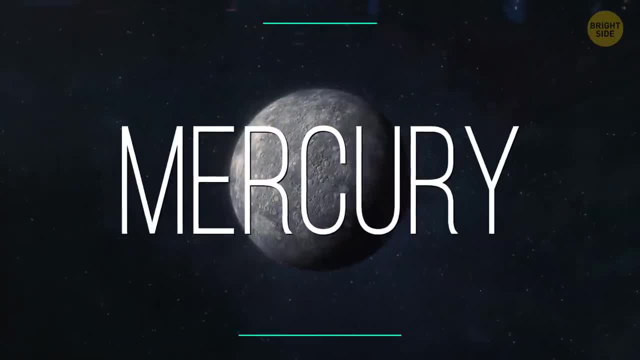 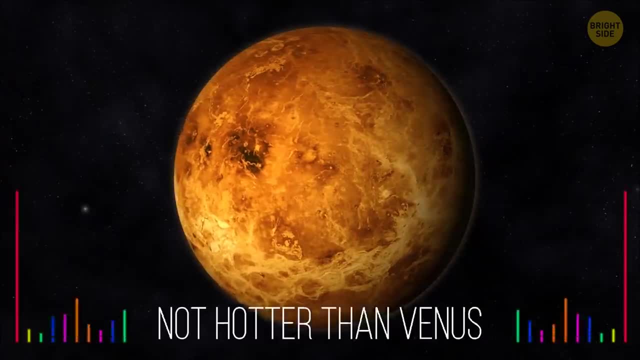 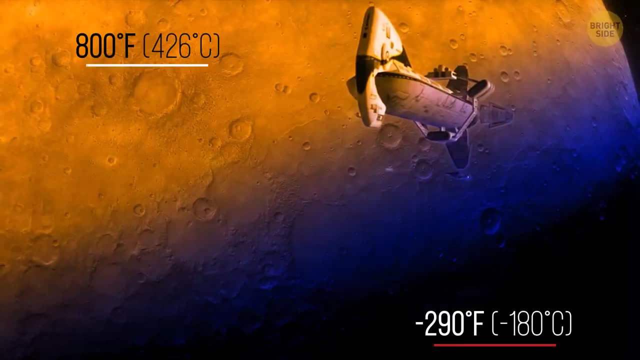 living on Mars might be totally normal. Living on Mercury would be really tough. It's the closest planet to the Sun and it's definitely hotter than Earth, But weirdly not hotter than Venus. It's really hot during the day, about 800 degrees, But at night it drops to negative 290.. 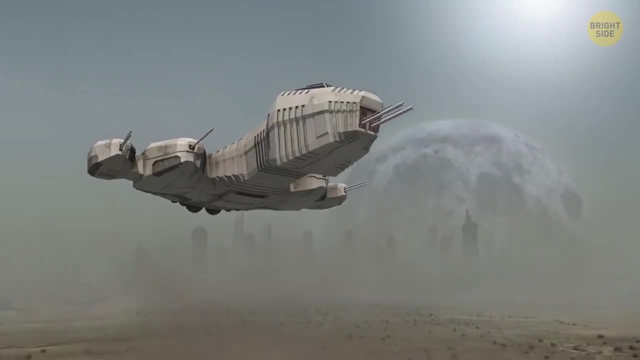 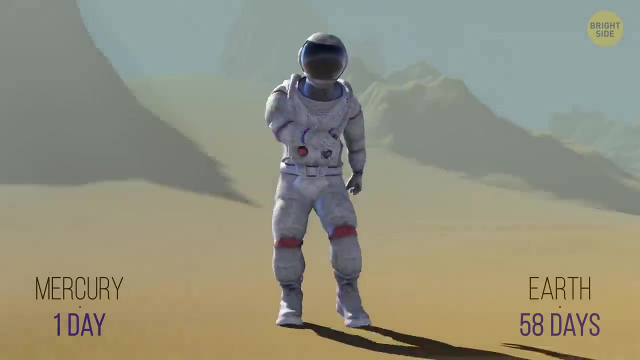 Days on Mercury are kind of crazy. You know when you finish the day, but you didn't really get a lot done. Problem solved: Move to Mercury. A day on this planet lasts about 58 Earth days. That means you'd have a lot of time to get ready. 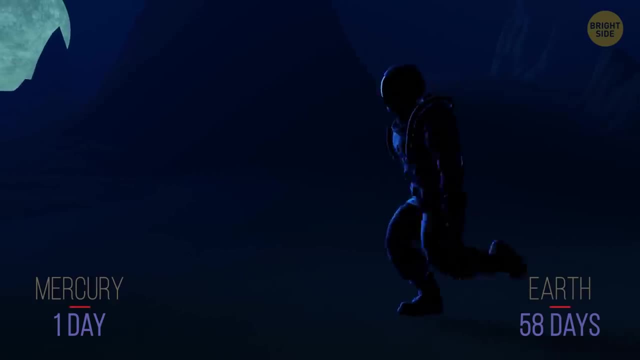 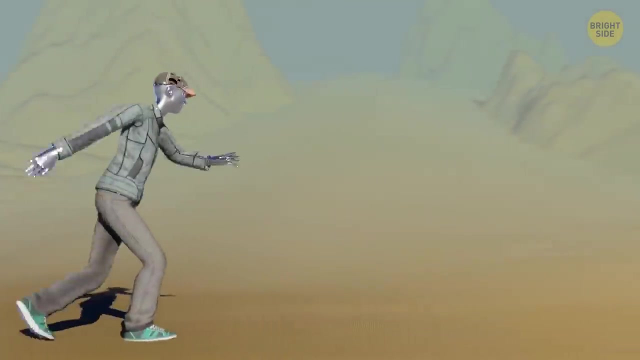 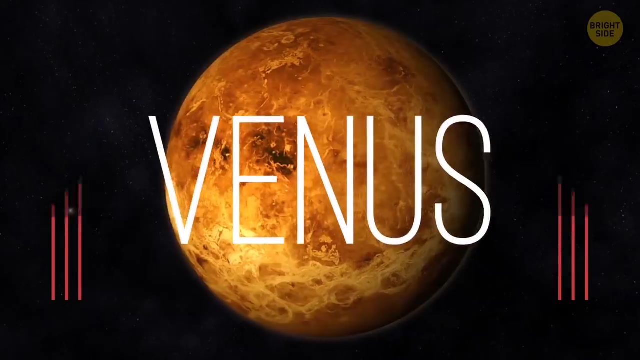 for bed. My guess, though you'd probably get kind of bored. One excellent solution: Somehow become made of metal Like titanium, nickel or platinum. Those guys can handle extreme conditions. Life on Venus would be way worse than Mercury or Mars. Pressure might be a tiny issue, You'd. 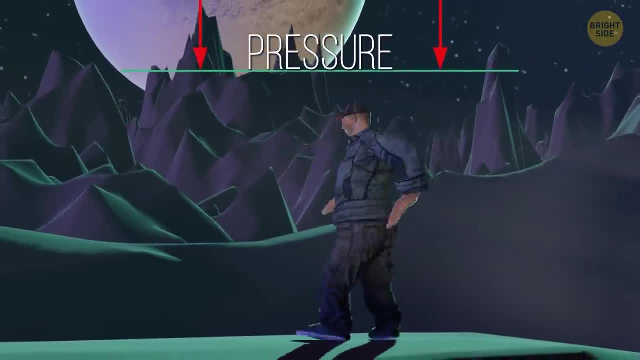 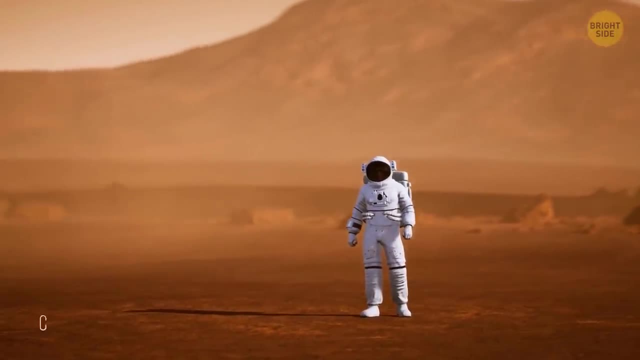 probably have one long, never-ending headache. Standing on Venus is like being 3,000 feet underwater. Oh, and that thing we need every moment of the day- Chocolate, I mean air. There's not a lot of that floating around on Venus. 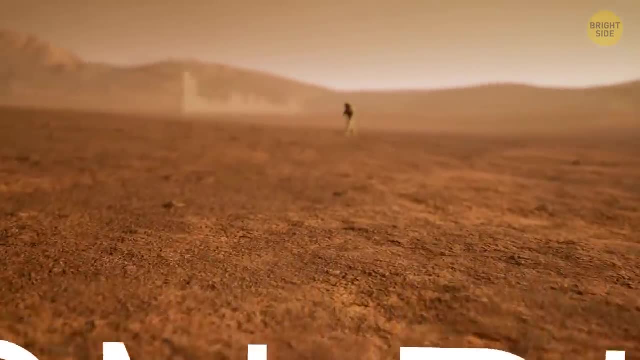 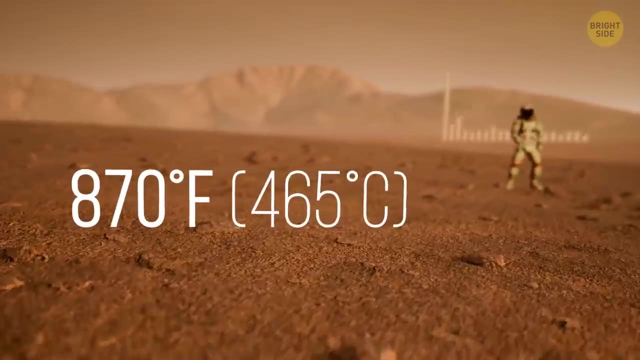 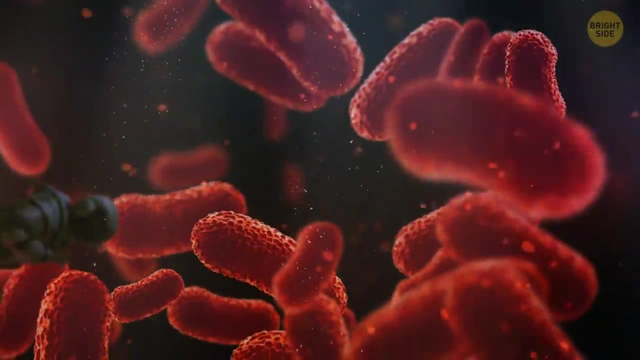 There's carbon dioxide everywhere And the planet's surface is completely dry. That means it's gonna be hot, 870 degrees hot. There are a few species on Earth that can survive the boiling point of water And maybe, if they mutated somehow, they'd survive Venus's crazy heat. 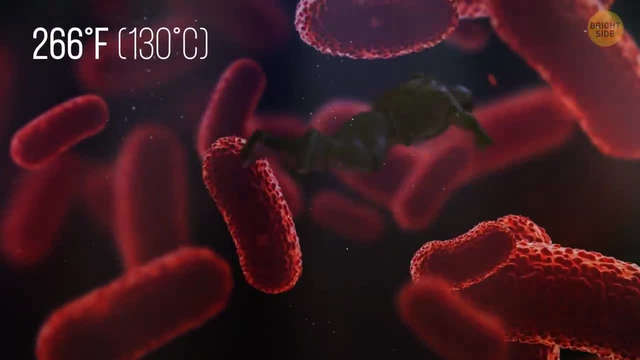 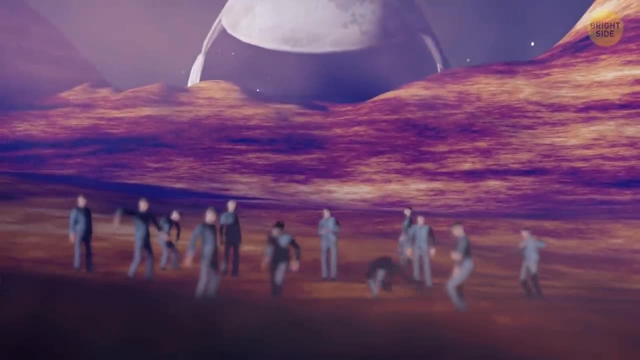 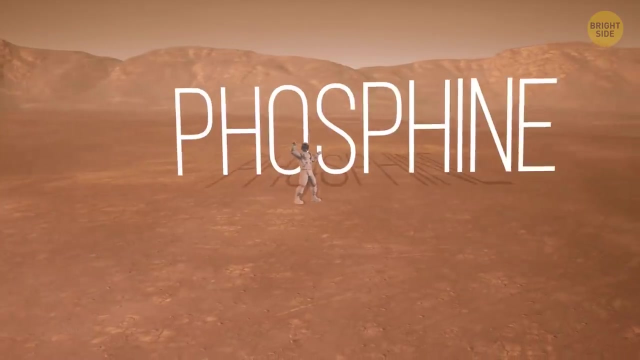 266 degrees is the record so far set by a species of microbes. So get ready for an epic body transformation. Want to live on Venus? You'd probably have to turn into a tiny microbe just to survive. Luckily, Venus's atmosphere has phosphine, which isn't great for humans, but microbes just love it. 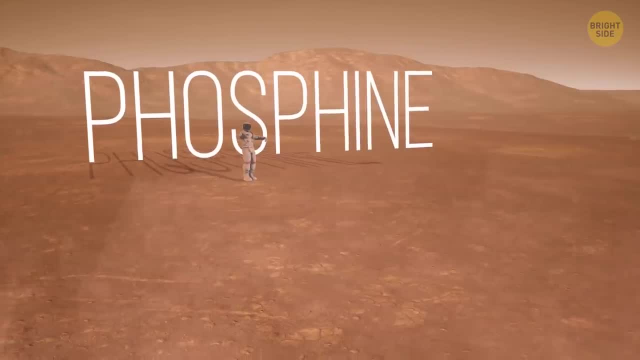 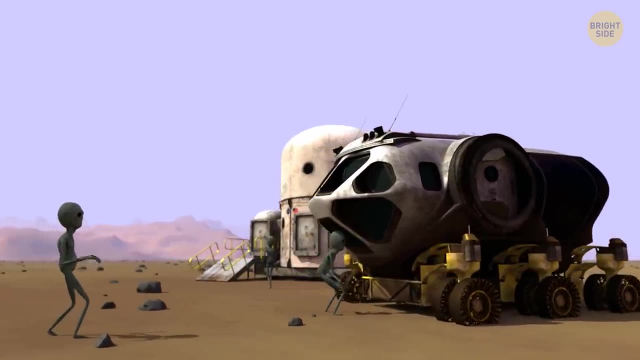 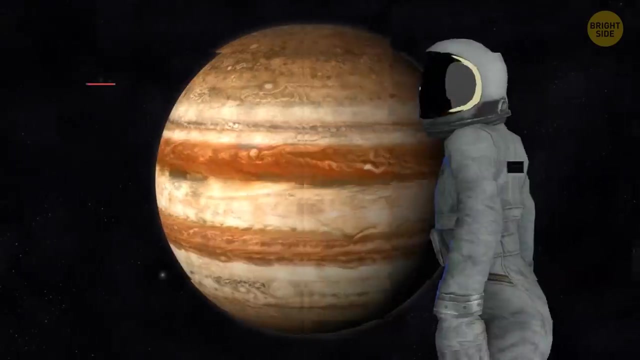 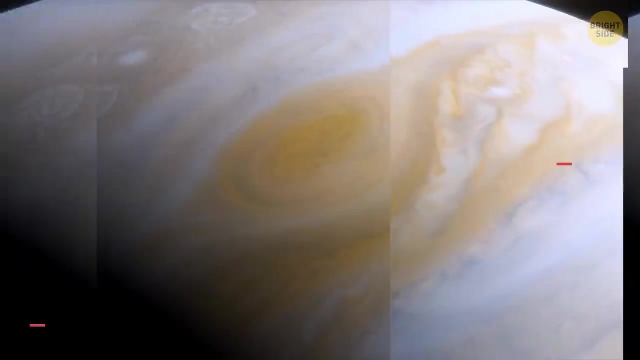 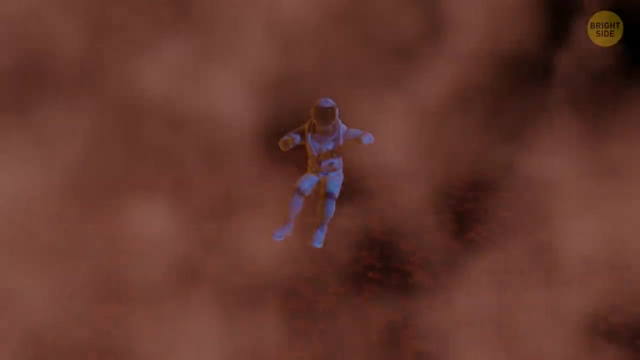 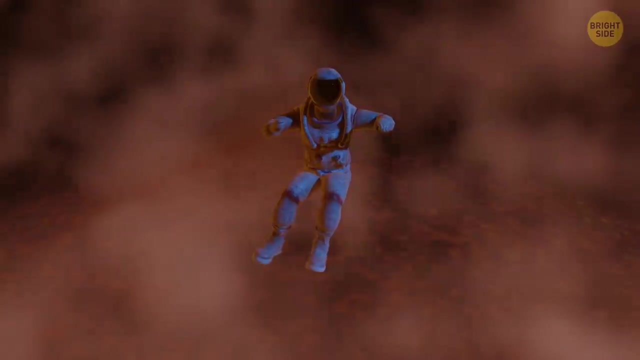 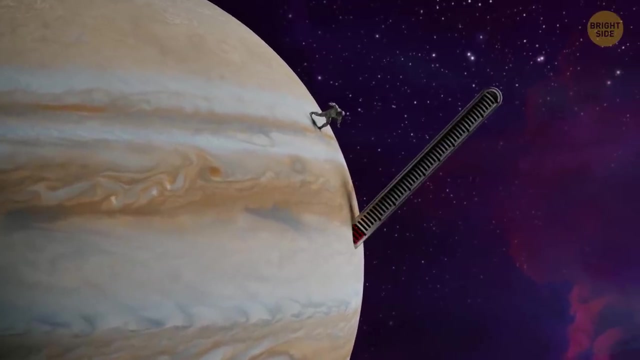 But since you're not a microbe- not yet anyway- you'd need to wear special gear to control the pressure and feed you air. It's not looking good. Maybe it'd be easier on Jupiter? Yeah, No, It's got no solid land. This planet's made of hydrogen and helium and is known as a gas giant. Unlike Saturn, you'd probably end up just floating around on it. It's like a giant cloud, And if you ever manage to land, it'd be like walking through a super thick fog. Temperatures fluctuate a lot here. It's freezing on the surface and the atmosphere can be super hot. The temperature can be super hot below the surface. We don't really even know. If you lived on Jupiter, there'd be no spoken languages. The gas planet absorbs radio waves, so even if you could speak, no one would hear you anyway And there'd be no music. so no dance parties. What's the point? 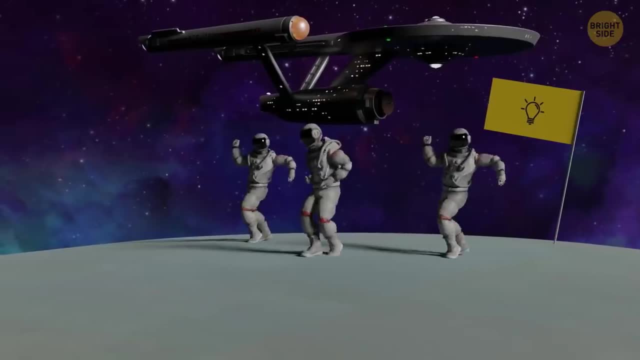 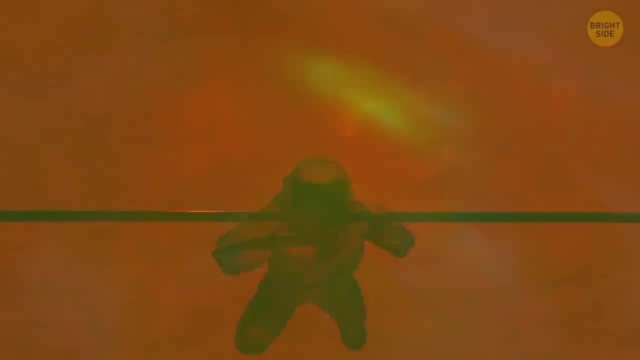 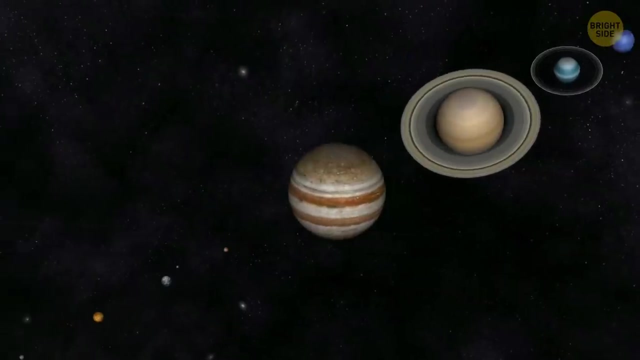 People would have to communicate in sign language. Great, But it's not. The atmosphere on Jupiter is wild: All kinds of winds and gas clouds. You probably wouldn't even be able to see anything, So that's not gonna happen. Still, Jupiter is awesome to look at. 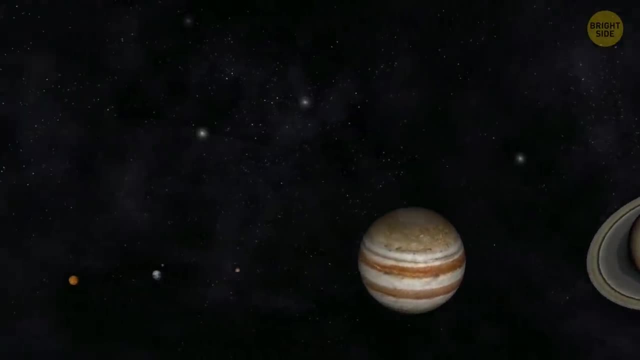 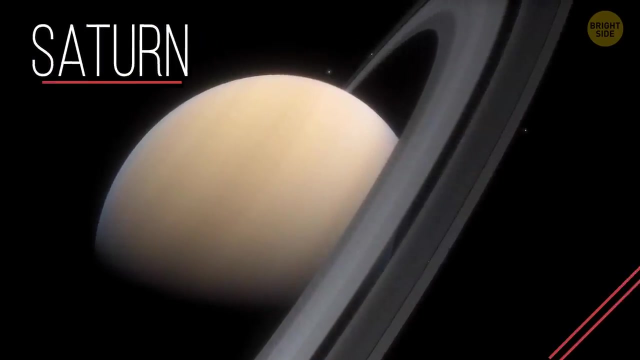 It's so big that it can fit all the other planets in our solar system inside it, with room to spare. A trip to Saturn will set you back about a decade, And it'd be a big ol' waste of time. Saturn's mostly made up of layers of gas. 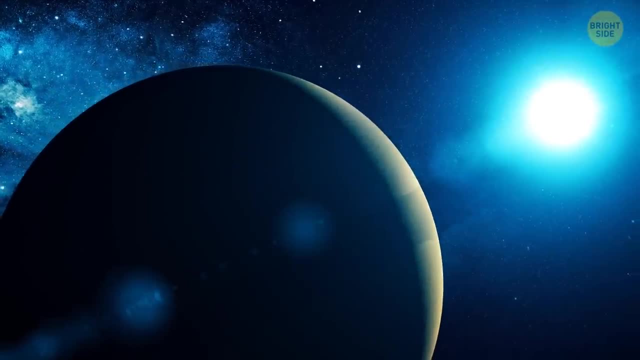 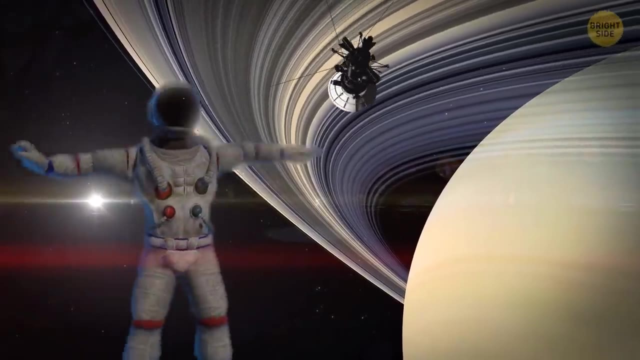 It has no solid surface, so farming, building or any other normal life would be a waste of time. But that's not all. Saturn's most powerful Earth activities are out of the question. Before landing on Saturn itself, you'd probably want to explore those iconic rings around it. 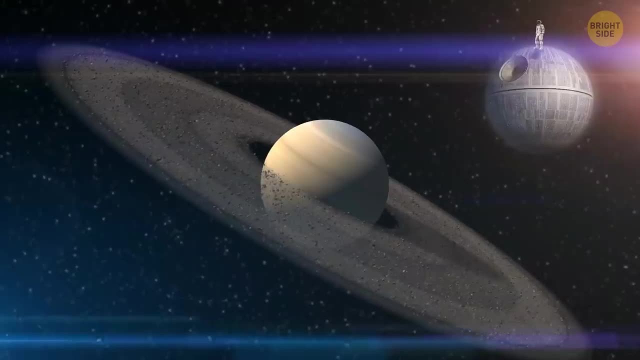 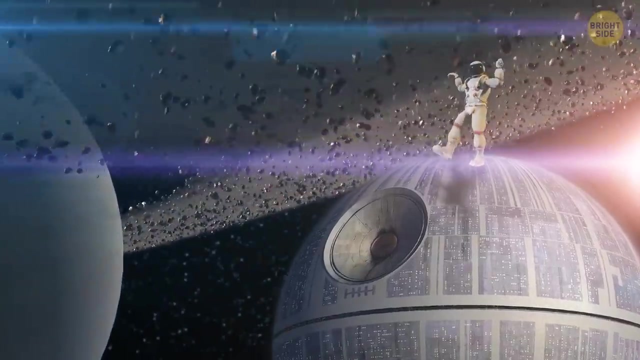 You'd fail, though, because the rings are made of millions of ice sprinkles floating in space. That's pretty hard to walk on. You might have thought that Saturn was going to be a good fit for you. Some layers of this gas giant's sphere actually have quite a nice temperature. 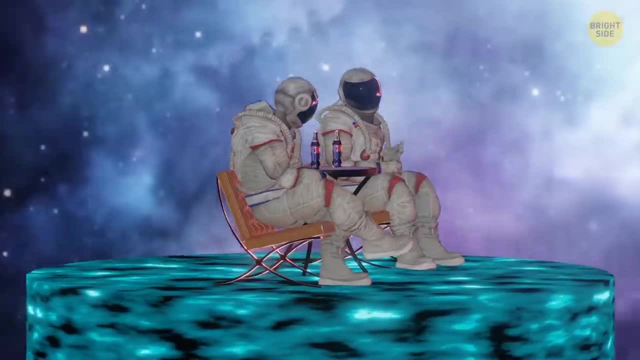 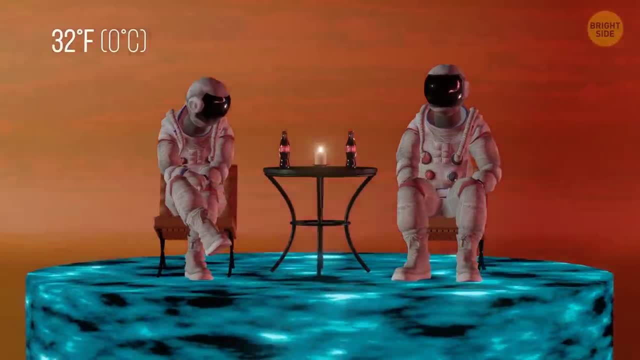 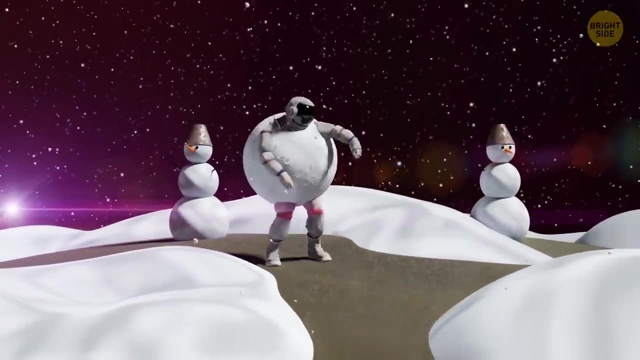 Northern Canada, Alaska, Sweden, Except that you can't walk on it. Anyway, it's only one minor layer. the rest of the planet is insanely cold, So I guess if you still want to live on Saturn, you've got some work to do. 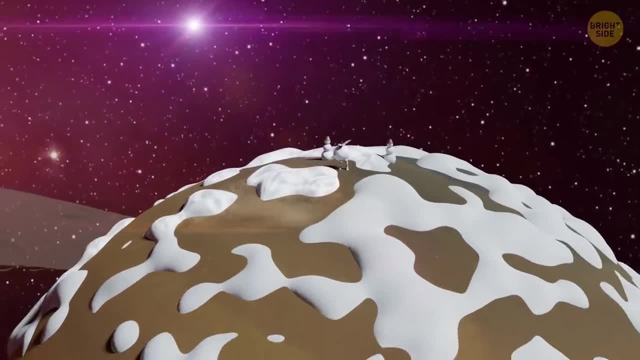 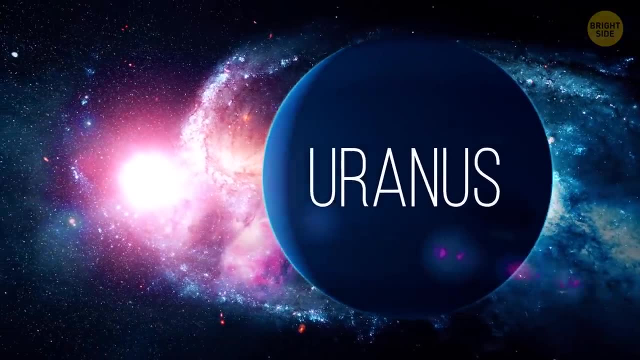 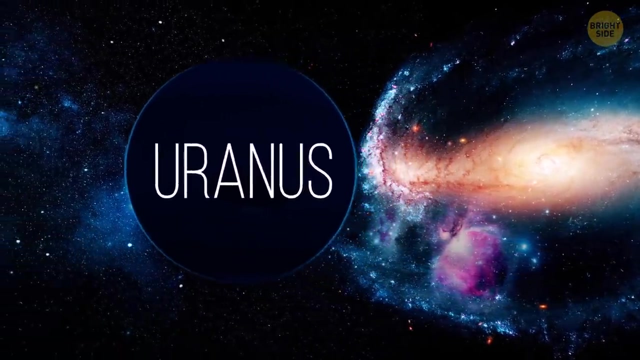 No biggie, you just got to turn into a snowball or something. What about Uranus? Time is kinda weird on Uranus. Time is kinda weird on Uranus. So if you're out that way looking for a nice vacation spot, definitely choose this planet. 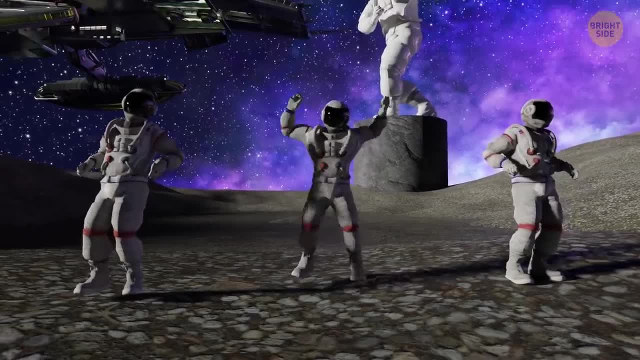 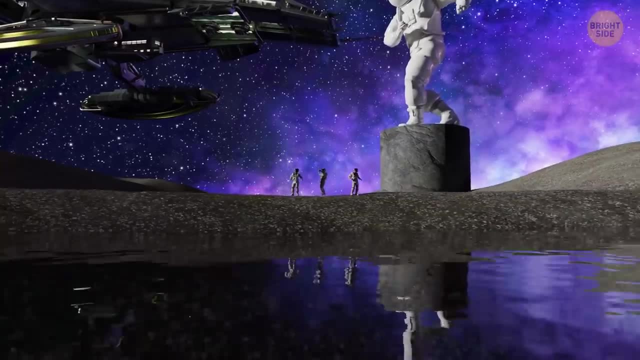 A two-week getaway on Earth lasts three years. on Uranus There's even a sea if you're up for a beach vacation. The only problem is that it's made of ammonia, that gross-smelling stuff they use for cleaning. But watch out where you land. 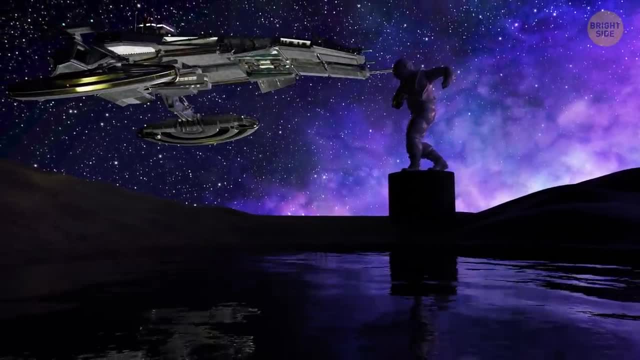 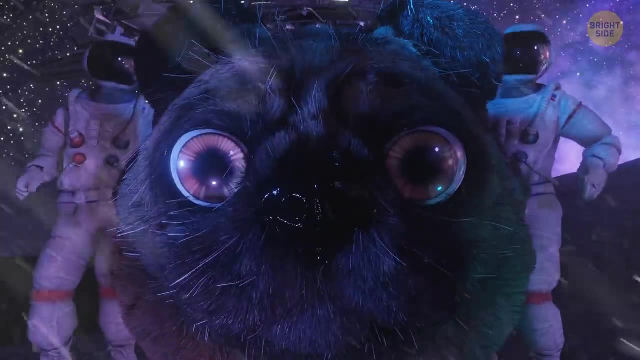 If you get it wrong, you might end up spending a whole year without any sun. How would you change if you had to spend a whole year in the freezing, dark Uranus winter? We'd need bigger eyes to see in the dark, plus more of that thicker skin to keep the cold out. 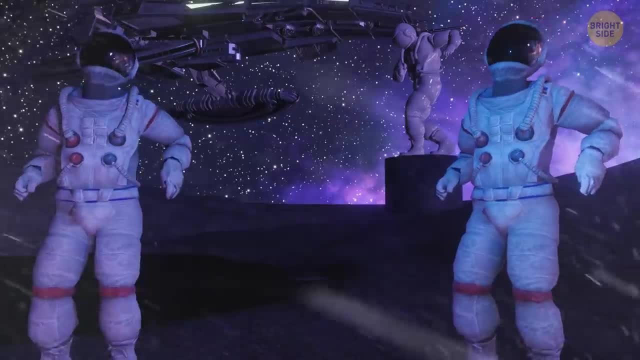 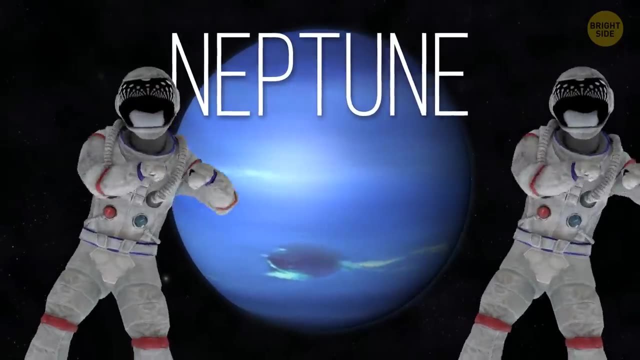 We might even develop a new hearing system, like dolphins have. Neptune: It's another gas planet, but scientists think there's probably a dense core inside. If you took the plunge to live on Neptune, you'd probably turn into a space reptile or cosmic fish. Endlessly, Endlessly floating around on the surface. Gravity on Neptune is just a little bit stronger than on Earth. Still, it'd be really hard to stay in one place. The wind there is super strong. You'd have to be much heavier to resist it. 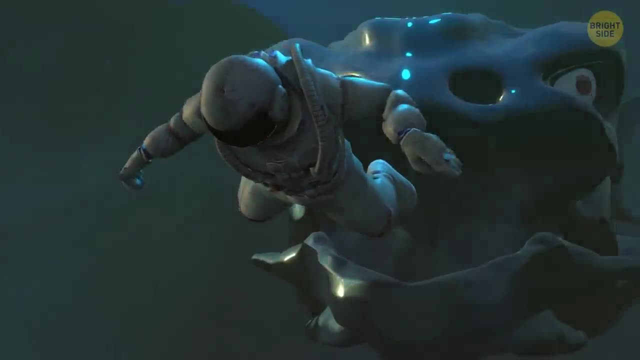 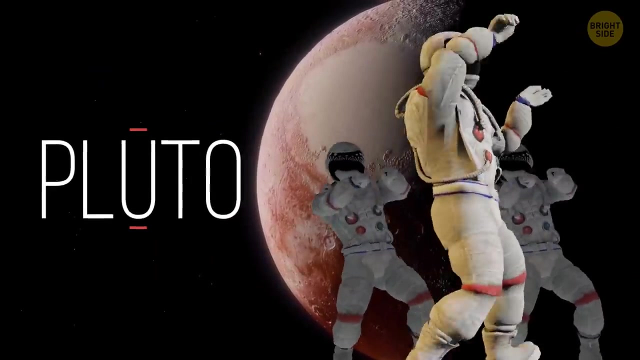 Time to eat again, Woohoo, But this planet's really impossible to live on. Scientists don't even want to send another spacecraft there. Welcome to Pluto. Freezing cold, tiny and super far away Doesn't sound too exciting. 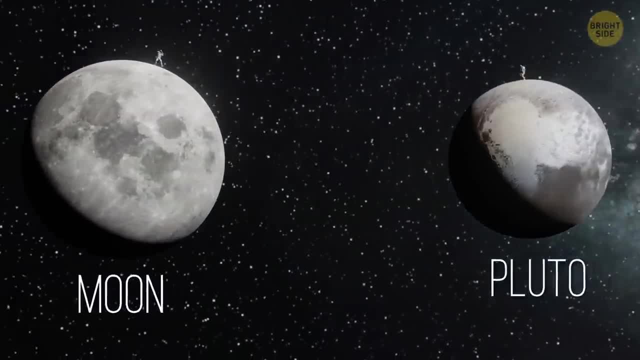 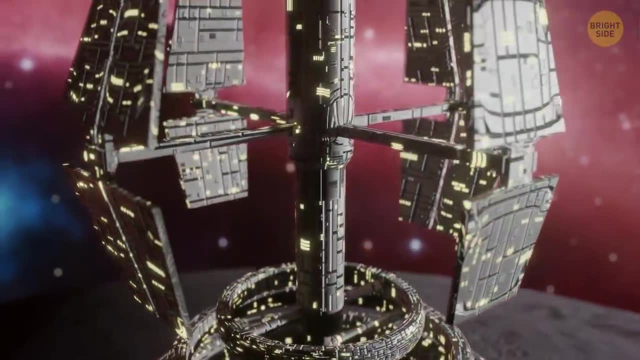 It's even special. It's even smaller than our moon. It would be so hard to stay on the planet. No more trampoline parks, people. You'd probably have to build yourself a huge machine that would spin you around, Sort of a fake gravity machine. 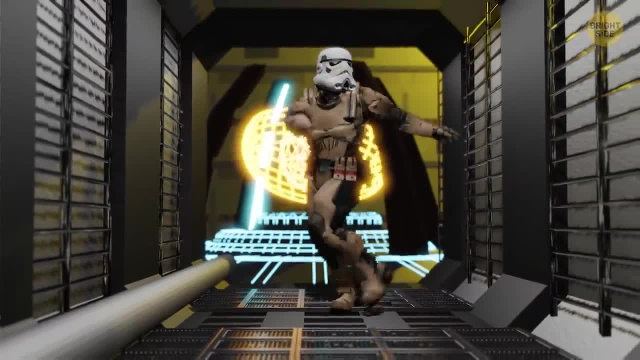 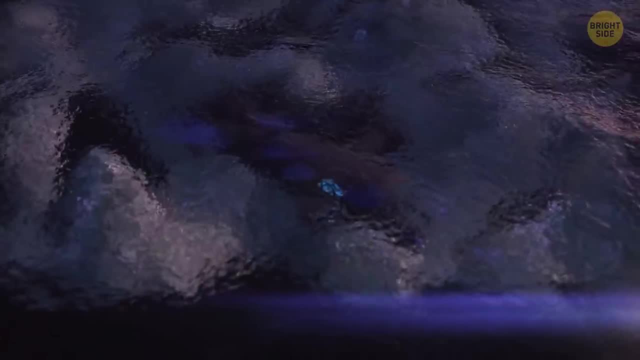 Still you'd try spinning around all day. You'd need a brand new nervous system to avoid feeling queasy all the time. But Pluto's not all bad. There's a liquid water ocean beneath the surface and ice mountains, If you got yourself a highly trained crew and a bunch of expensive gear.